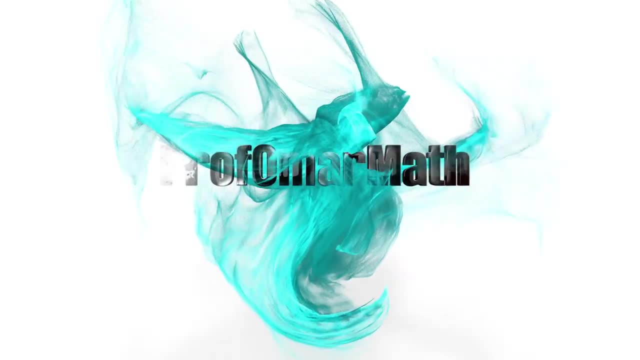 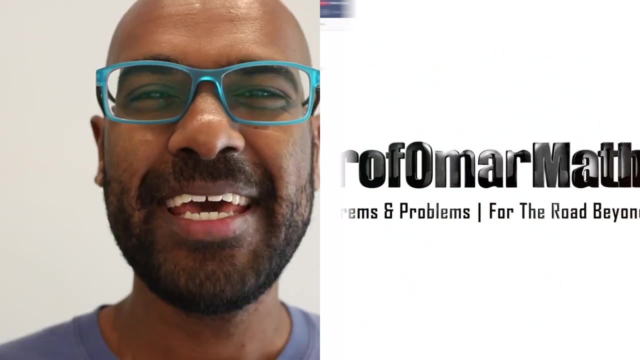 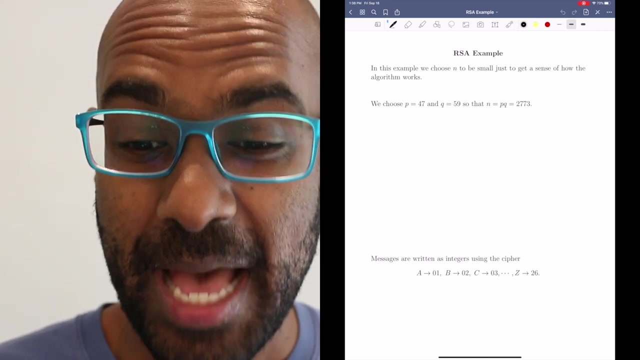 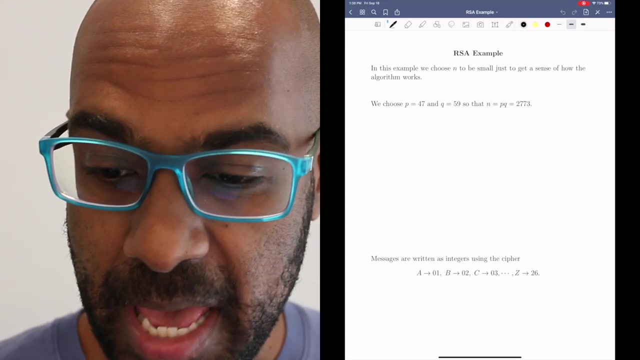 Hey, welcome to today's video. I'm Prof Omar. Today we're going to run through an actual example to see how the RSA algorithm actually works. In this example, we're going to list out all of the pieces of the algorithm and we'll see how sending a message involves this. 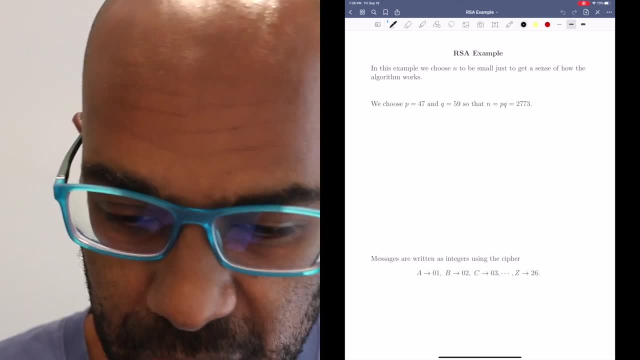 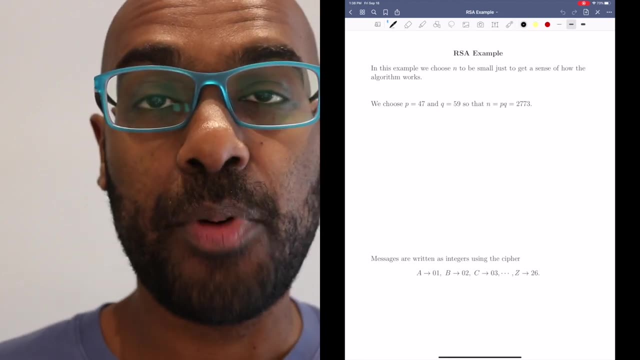 encryption and then the decryption process. We'll see the entire process throughout. Okay, so one of the things the algorithm required was a number n, that's a product of two very large primes. So we're going to pick primes that are reasonably sized, just for the illustration. 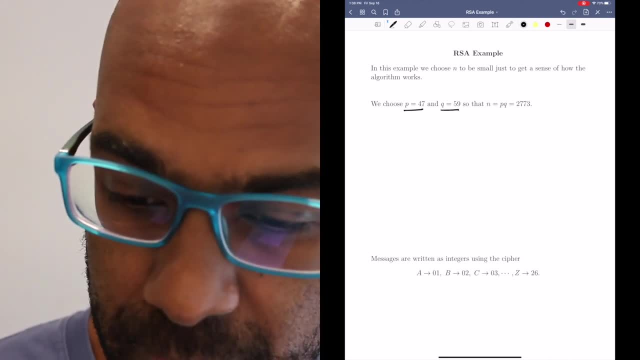 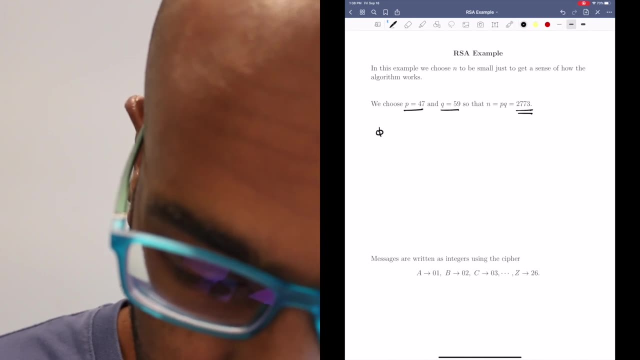 purposes, We're going to pick 47 and 59. So the product is this: n, right over here. Okay, so one of the things we're going to need in the algorithm is 5n. We talked about in the previous video that 5n is p. 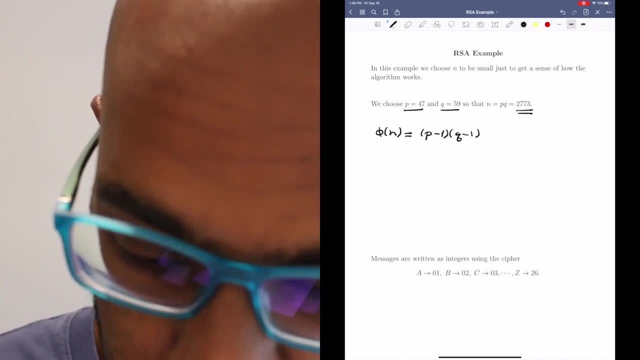 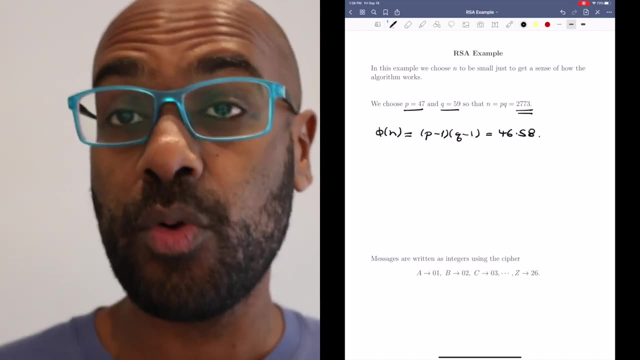 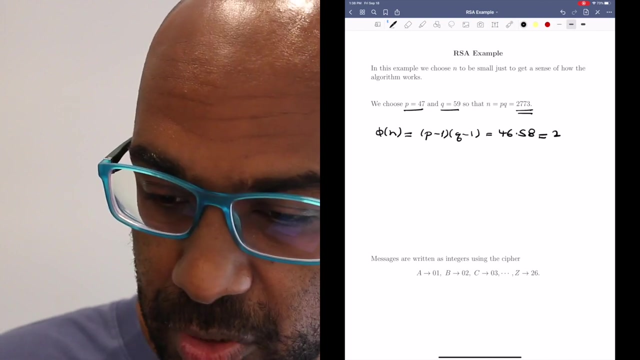 p-1 times q-1, which in this case, then, is going to be 46 times 58. And we're going to use this number quite a bit throughout the algorithm so that we know what we need to do for our modular calculations. So this number turns out to be 2,668. 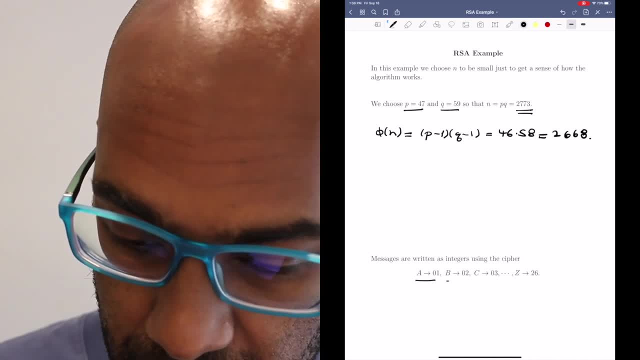 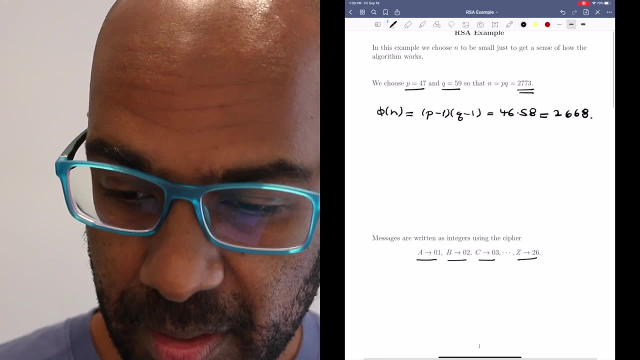 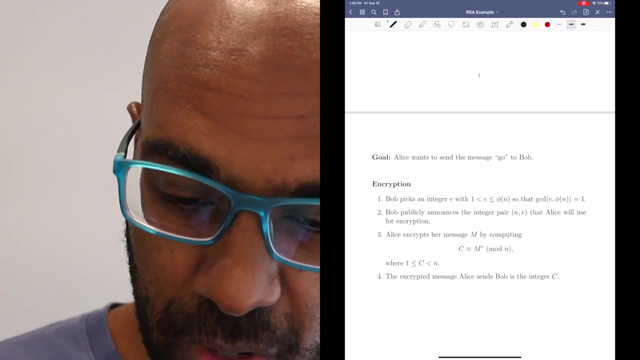 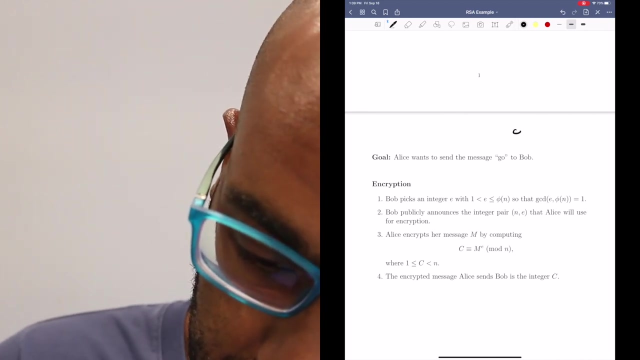 And, as usual, any message is going to use the cipher where any letter corresponds to its position. Okay, so let's jump in and actually try this out. So our goal is going to be for Alice to send a message go to Bob. So here is Bob and here's Alice. 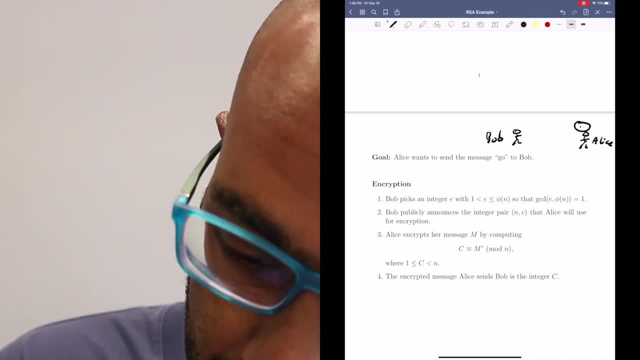 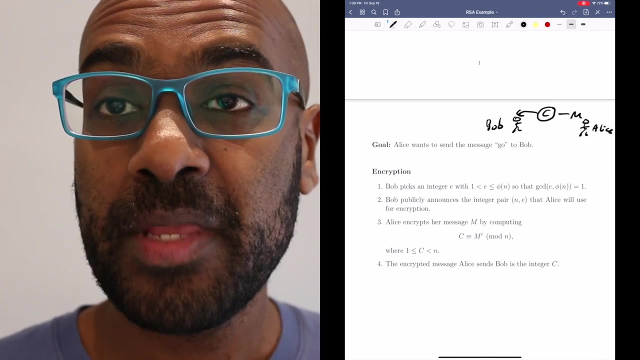 The first thing we need to do is take this message that Alice has and change it to something secret. It's going to be a secretive that we send over the public channel to Bob. That requires some pre-processing by Bob, And we're going to see exactly how that's going to work, Okay. 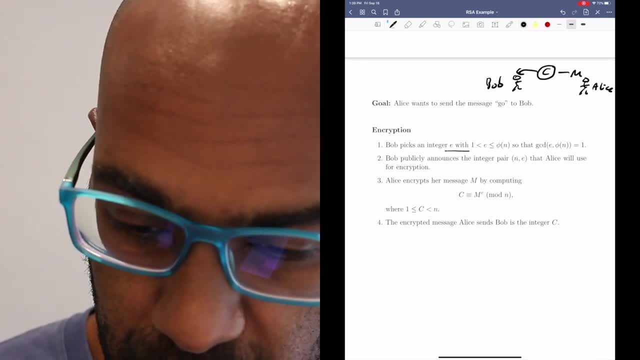 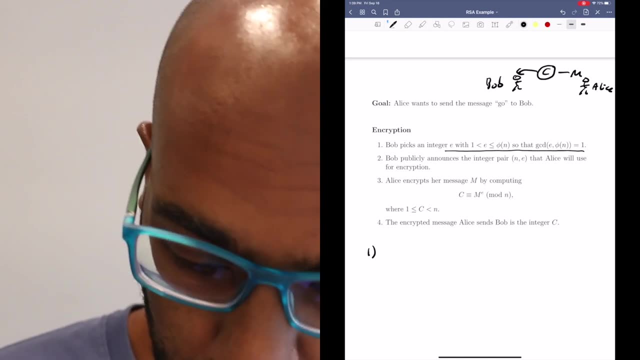 so the first part is that Bob needs to pick an integer e that satisfies this condition right over here. Okay, so how are we going to do this? So we saw a little bit earlier that Bob knows that 5n is 2,668. 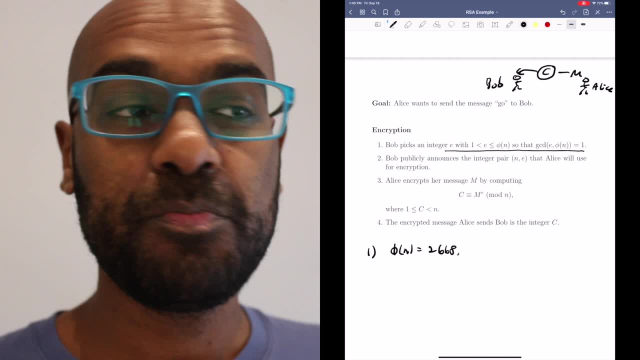 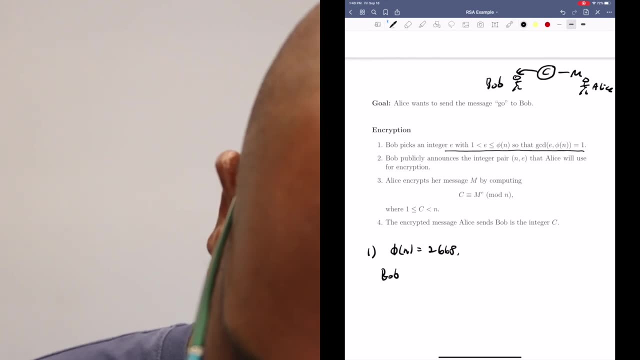 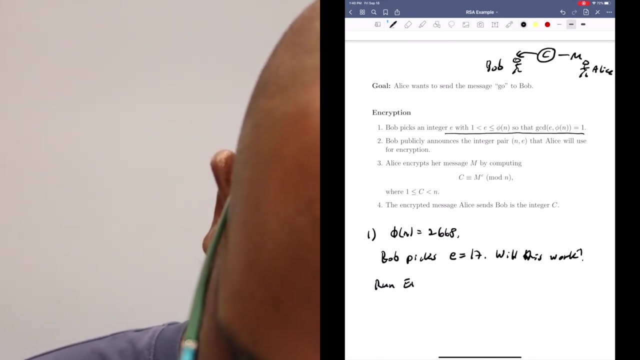 So what Bob can do is pick random values for e and test things out. So let's say Bob picks e randomly to be 17.. Will this work? Well, we can test using the Euclidean algorithm. So run the Euclidean algorithm on the pair. 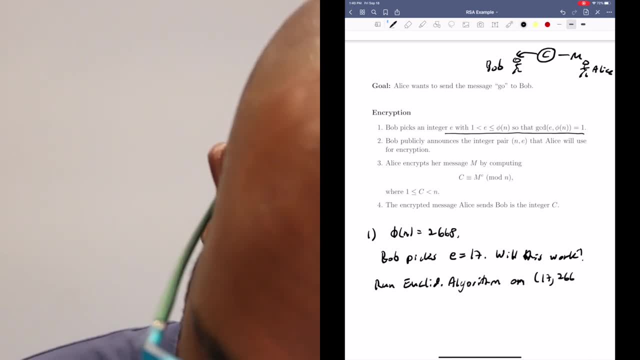 of numbers 17 and 2668.. Okay, so we're going to run the Euclidean algorithm on the pair of numbers 17 and 2668.. Okay, so we're going to run the Euclidean algorithm on the pair of numbers 17 and 2668. 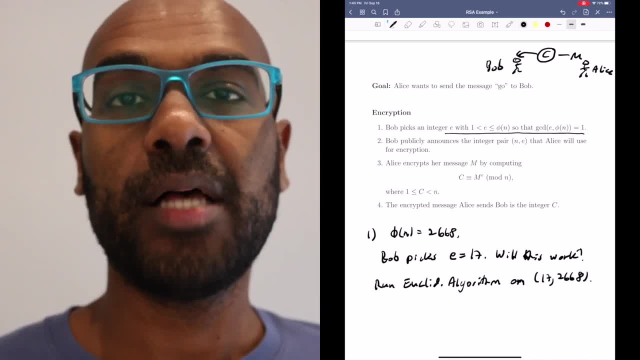 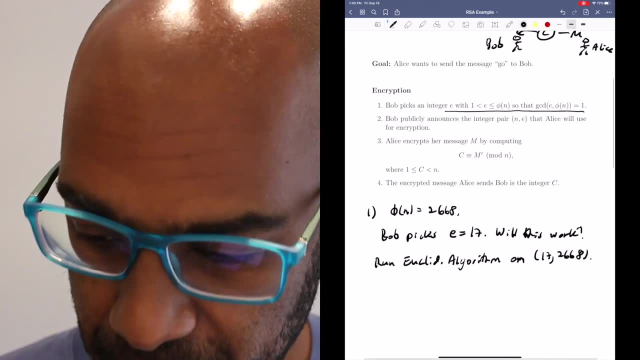 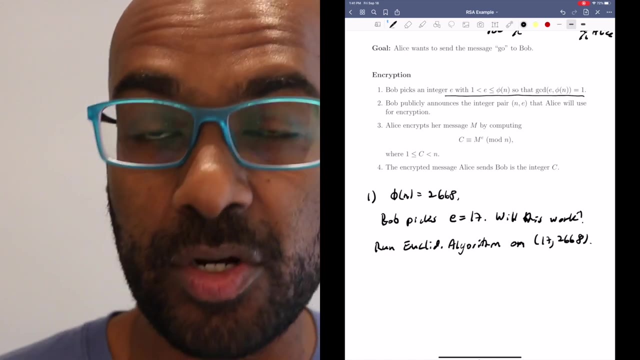 we're not going to illustrate running that process here, but if you want to see how that process works, check out this video right over here where we talk about the details. Okay, so if you do that, you can actually figure out a way to write one as a linear combination of these two numbers with integer. 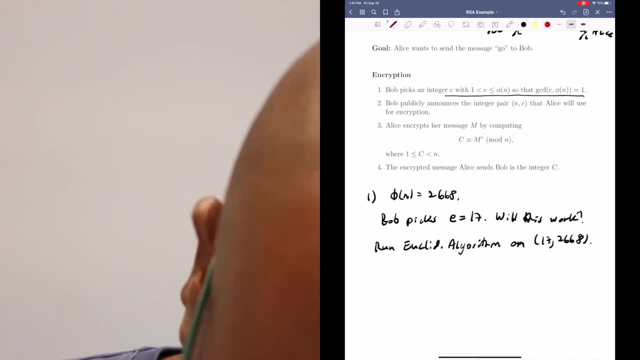 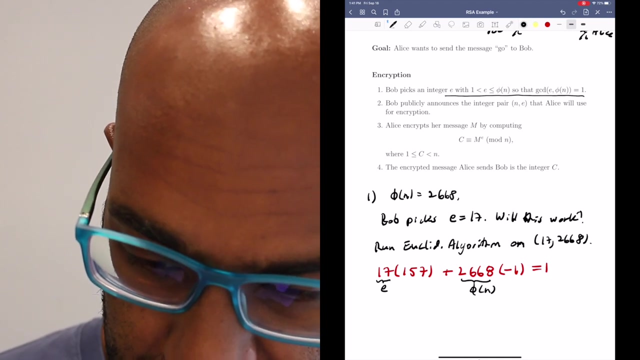 coefficients and it turns out that 17 times 157 plus 2668 times negative, 1 is 1.. So, to emphasize again, this number here is e and this number here is 5n. Okay, so we have e times some number is 1 plus a multiple of 5n. 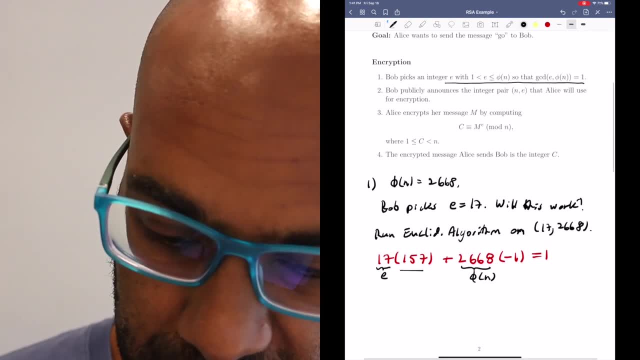 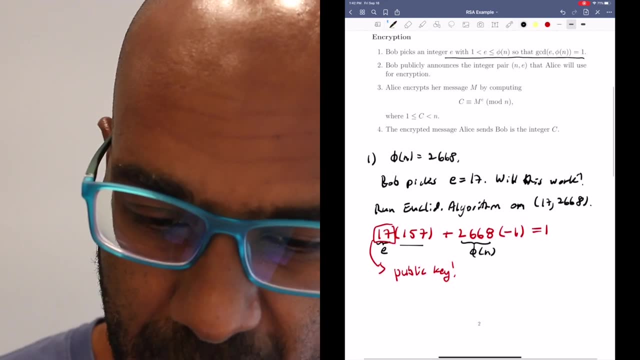 Okay, so we have e times. some number is 1 plus a multiple of 5n. That's great. Okay, so our public key then is going to be 17.. Okay, and that's what we're going to send publicly to the entire channel. Okay, so now what we need. 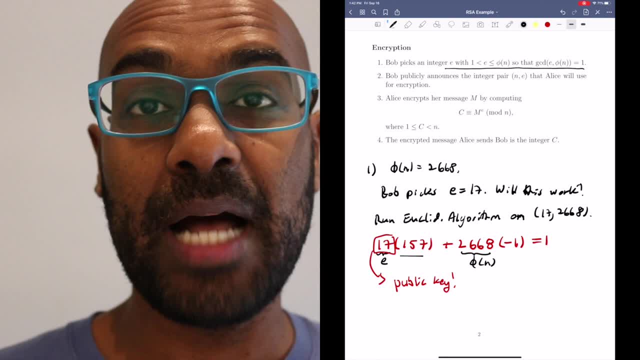 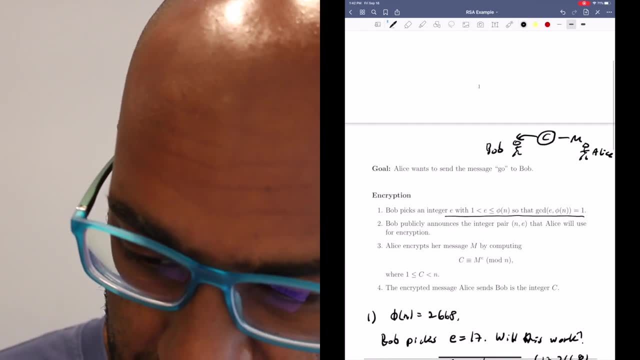 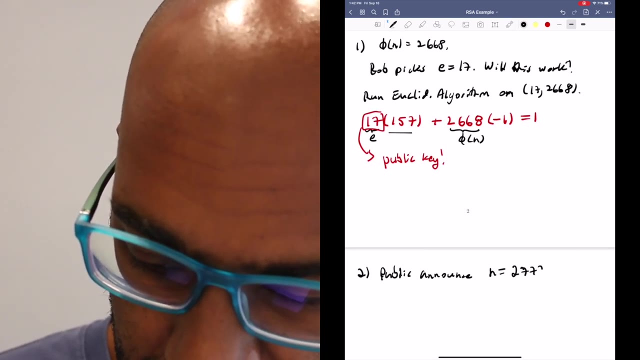 to do is publicly announce this. That's fine. So Alice has this pair publicly announce that n is the number that it is, which is 2773.. So you can imagine if you didn't have a calculator, 2773 is a hard number to know those prime factors of And in general, if this 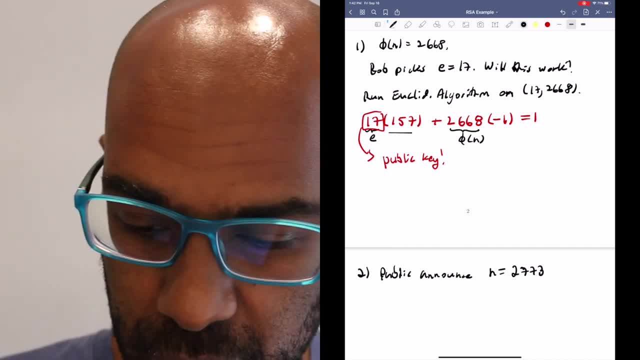 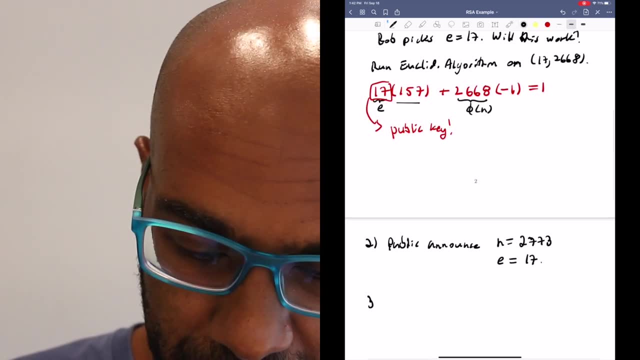 number was really massive. computers can't even do a good job of figuring out that. And then e is 17 is going to be publicly announced as well. Okay, so this is stuff people need to do work. So now Alice is going to do some work. She's. 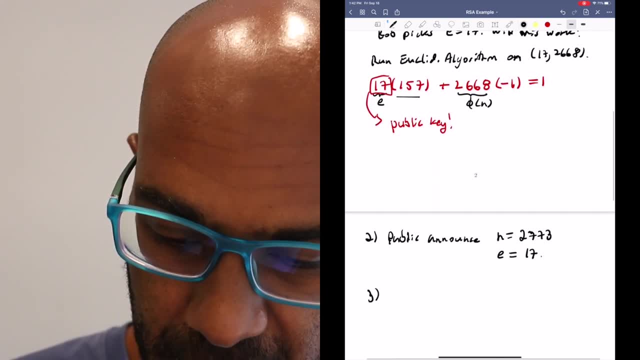 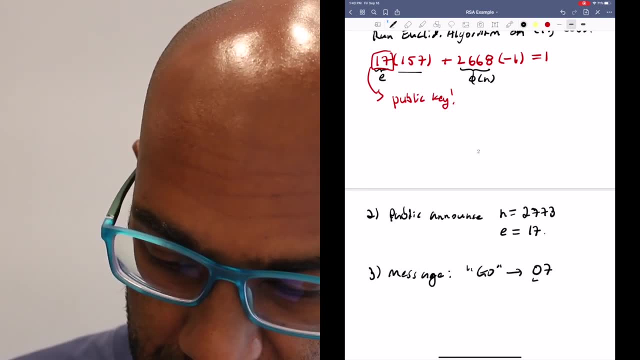 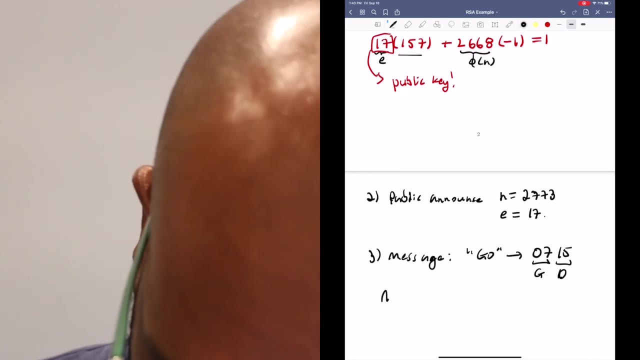 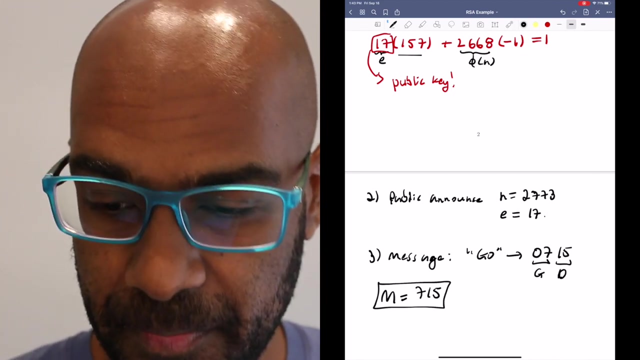 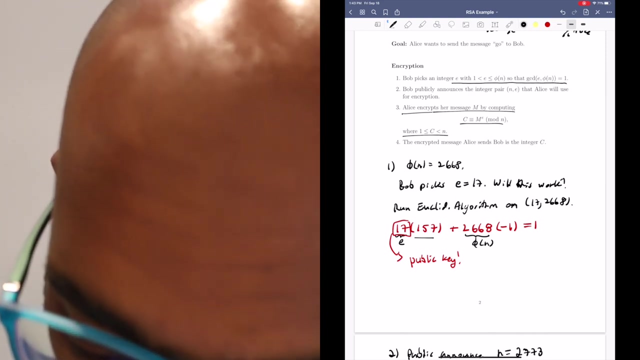 going to take her message and encrypt it. So the message was go. g is the seventh letter of the alphabet, O is the 15th, So m. the message that Alice wants to send is 715.. And according to our instructions, we want to compute 715 to the e mod n, So we need. 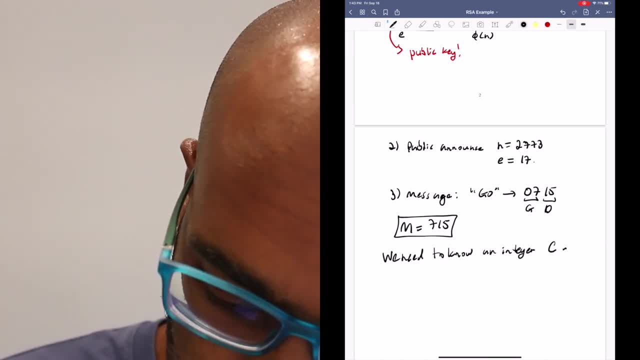 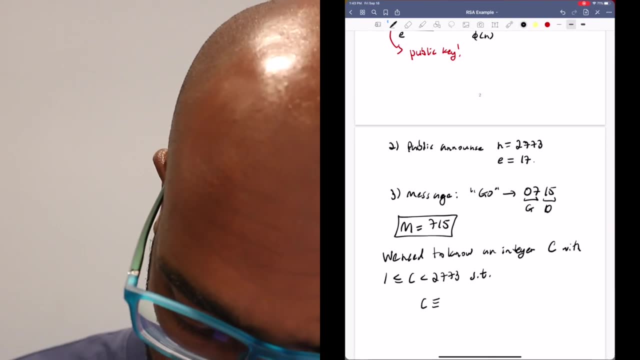 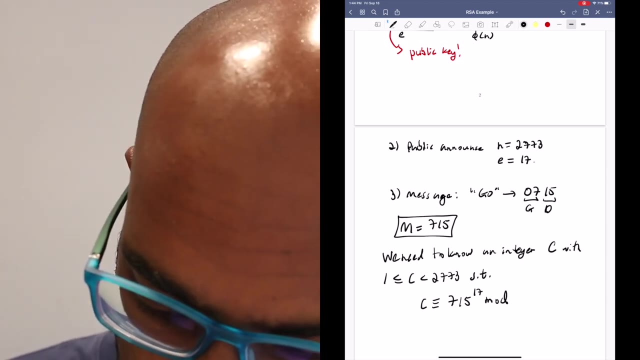 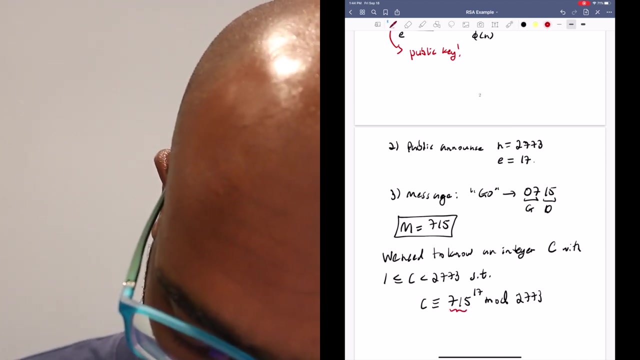 to know an integer c, with c being between one and n, so that c is congruent to m, to the e, which is 17 modulo n 2773.. Okay, so I want to emphasize this thing. here is our message: m, this is our encryption key. e and this is m. 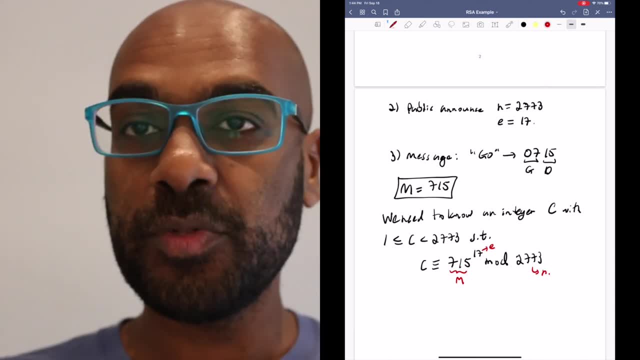 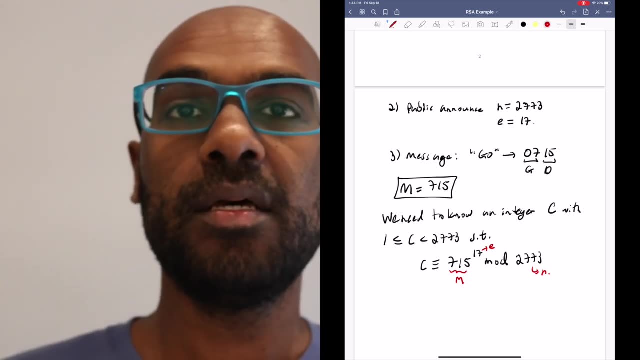 okay. so this takes some work and there are a lot of different things that we can do. we can start raising 715 to small powers like 2 and then take that result and square it to get 17 to the 715, to the 4, etc. etc. 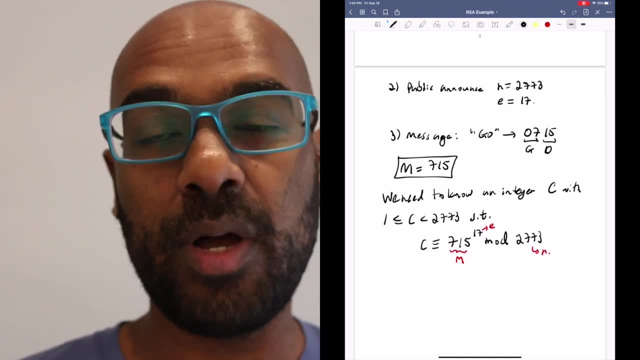 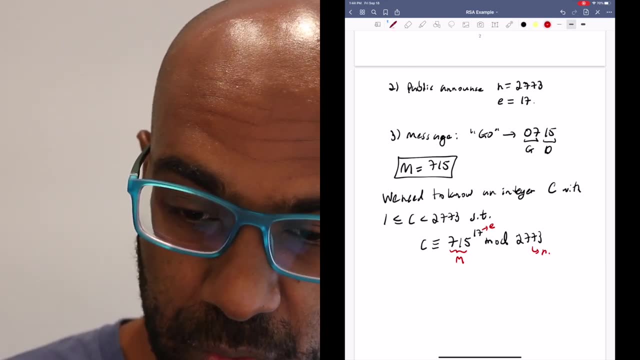 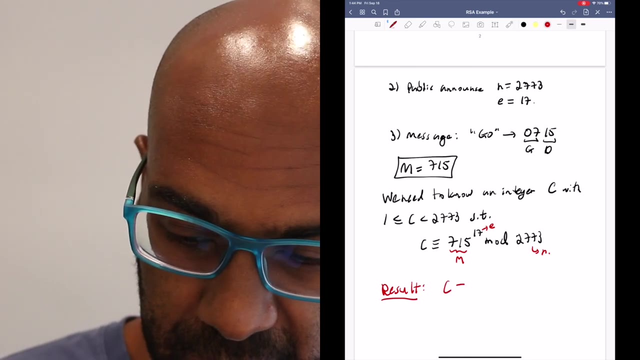 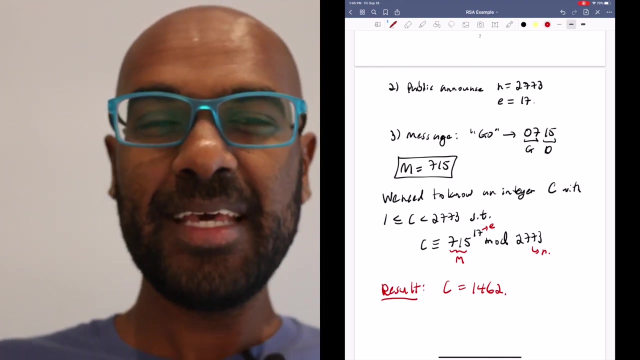 and lots of other techniques. if the number e was, like, quite large, we have other techniques that we can use as well, that we've learned in previous videos. okay, so if you do this process, i'll mention what the result is. the result is that c is going to equal 1462.. cool, okay, so this 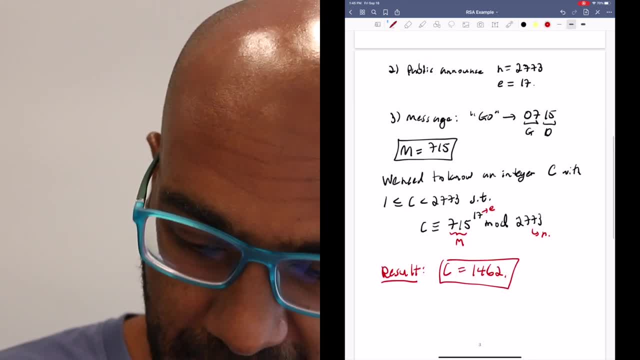 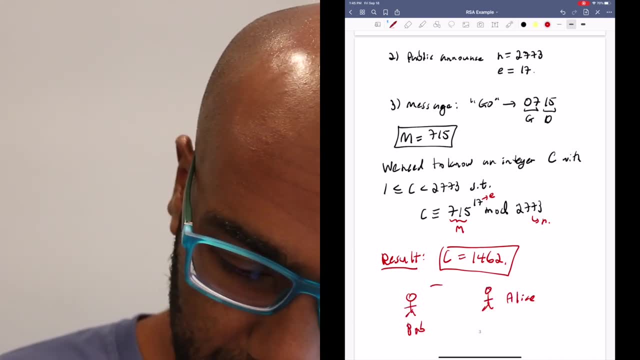 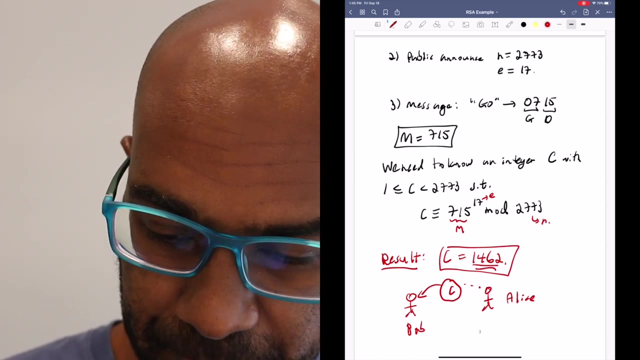 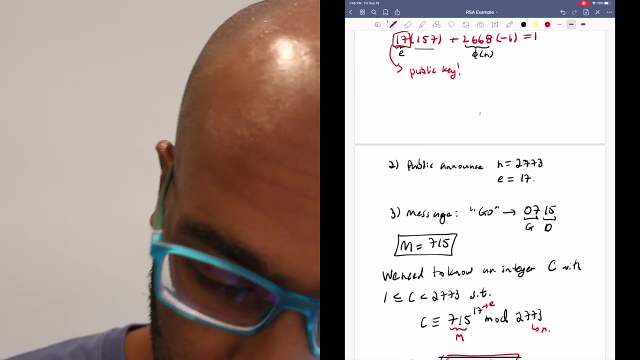 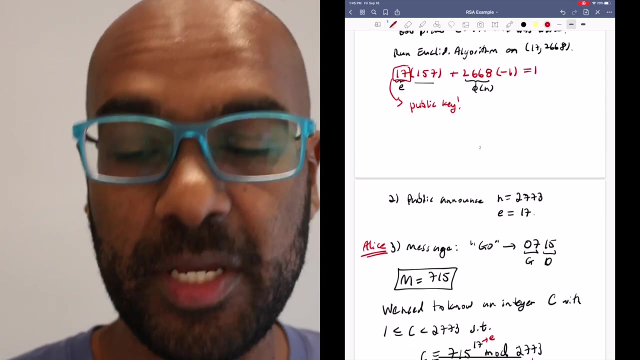 is the thing that bob is going to receive. so here's bob, alice, and the message that bob is going to receive is this encrypted number c right over here. okay, so that's the end of the encryption process. this is all work that alice does in number three. given all the public information, 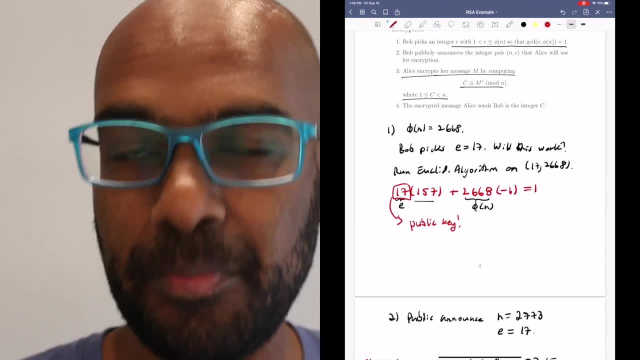 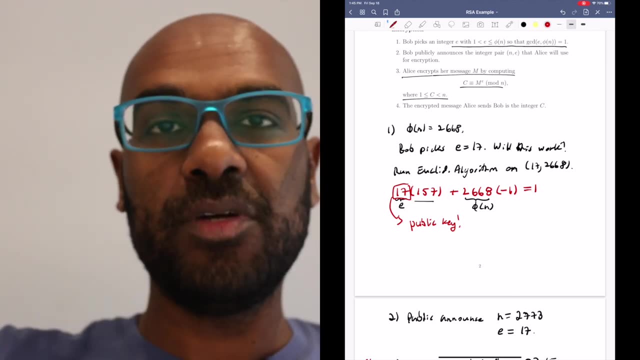 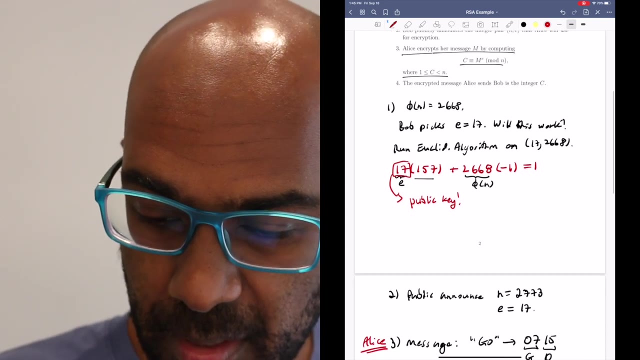 so, if we think about this overall, what's happening is: bob announces n and e as a bound on the length of the numbers that bob is allowing to receive, and then e is a special encryption key that he's sending publicly for people to send messages with, And so Alice's job is to 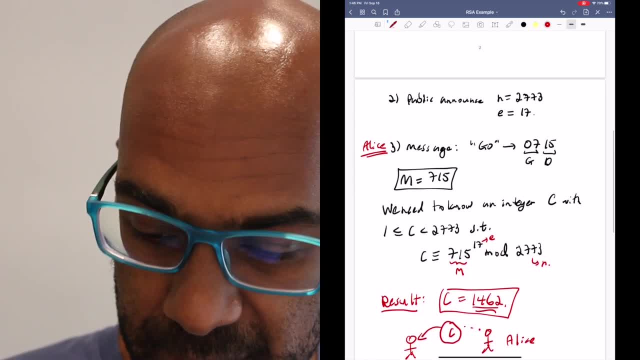 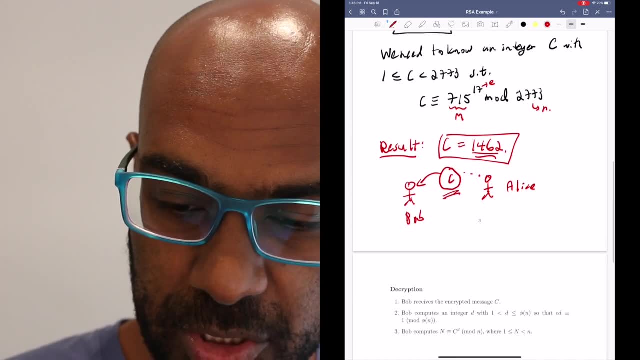 take her message that she wants to send and encrypt using this process. Okay, so now that Bob receives this, what he really wants is the original message. If Bob tried to use the cipher to figure out what 1462 was, he'd be like okay. 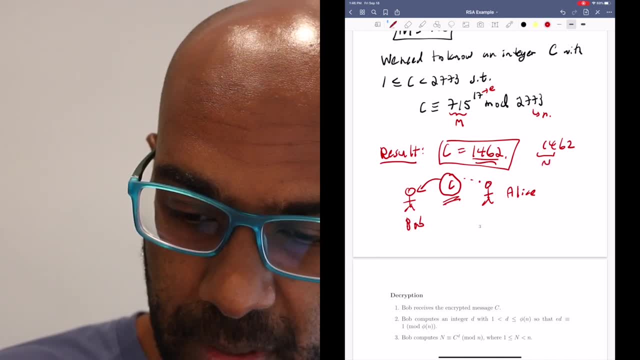 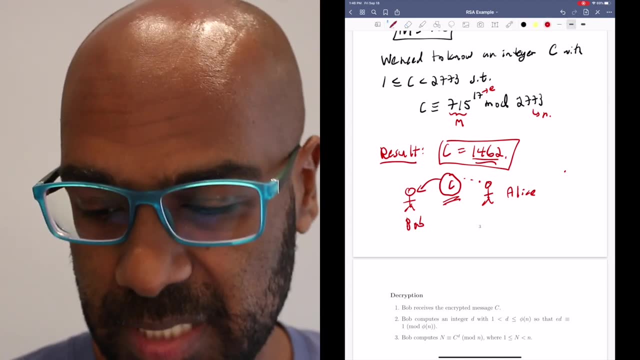 what's the 14th letter of the alphabet? Maybe it's N, And then the 62nd letter, Question mark, Not clear, So anybody who tries to intercept and figure this out will have no luck. Alright, that's okay, though, because Bob has a process. So, Bob, 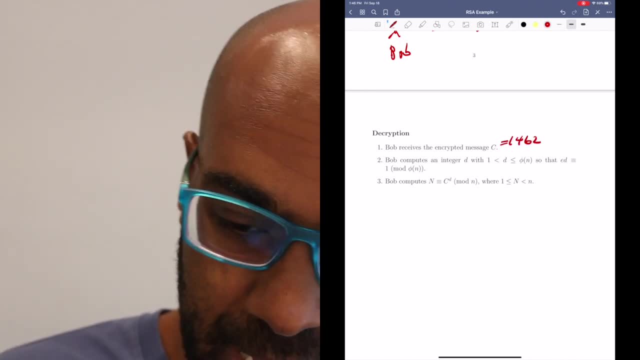 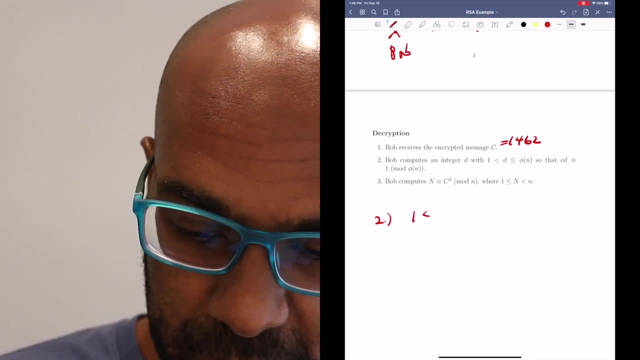 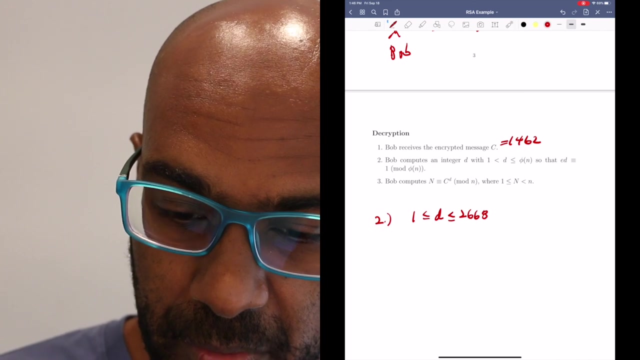 receives the C, which is 1462, and then he has to do some work. The first piece of work that Bob needs to do is compute an integer D so that 1 is between D and this phi of N, which we computed to be 2668.. Alright, with the condition that 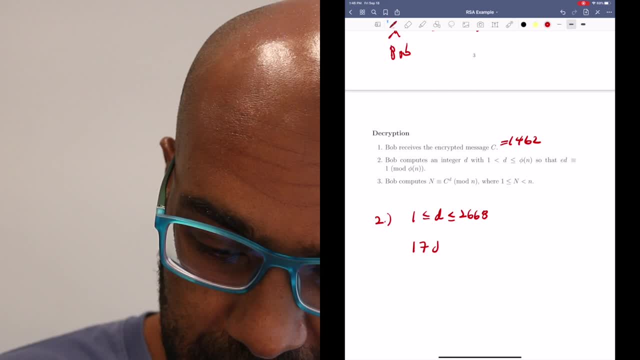 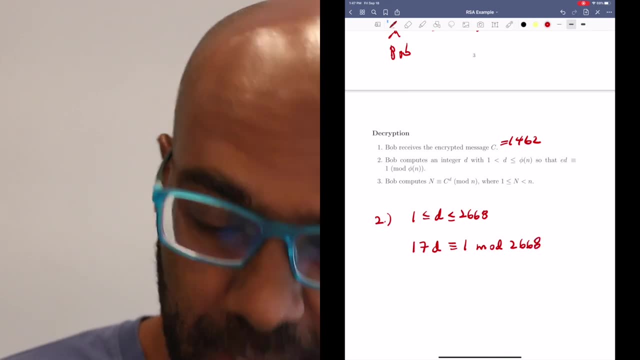 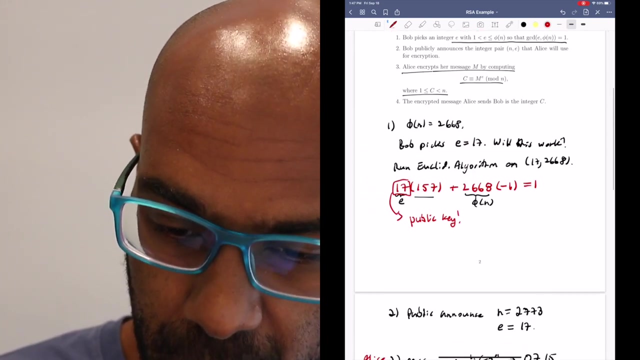 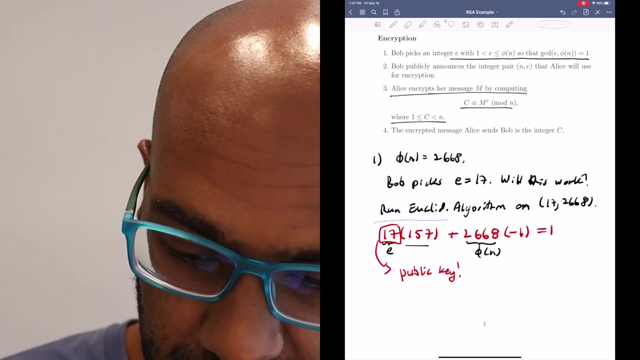 ed, so that 17 D is congruent to 1 mod 2668.. Now, luckily, Bob actually did this work already. If we go back here, Bob computed this interesting integer combination using the Euclidean algorithm. One of the things that's convenient. 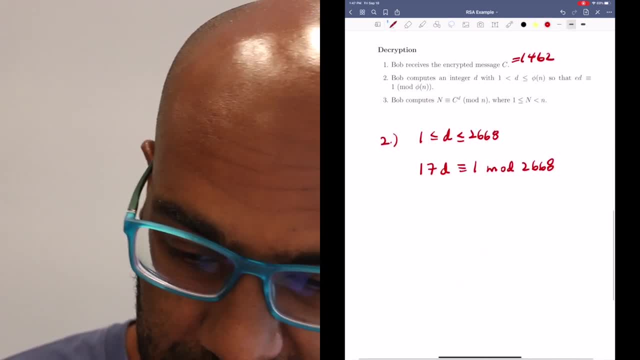 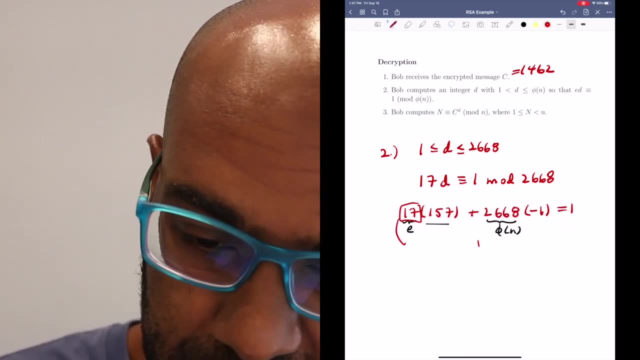 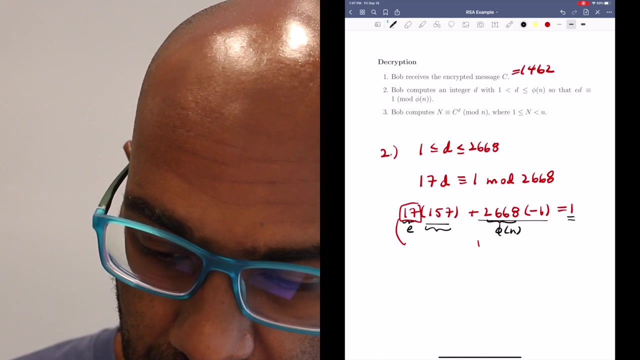 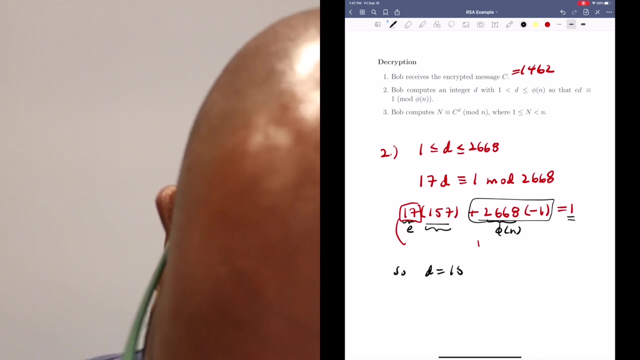 about this it is that it actually addresses this question as well. If we look at this integer combination, it tells us that 17 times this number is 1, plus a multiple of 2668.. So he's already done this work. actually, d equals to 157. 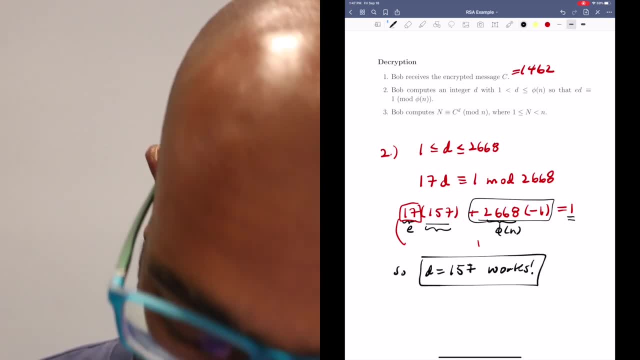 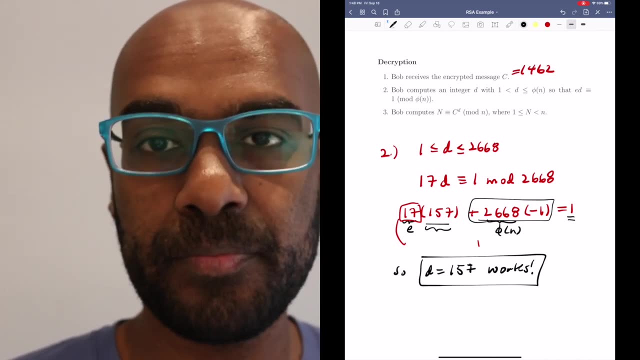 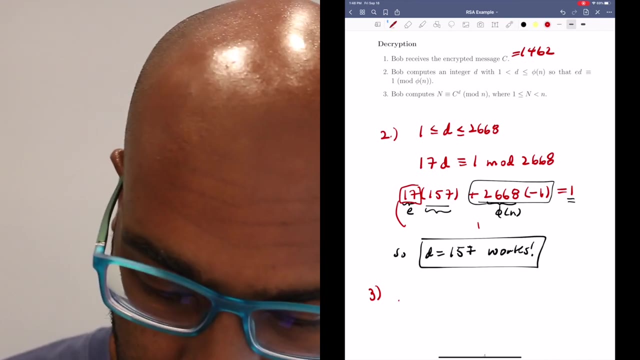 works as a number that we can use. This is convenient, so Bob doesn't have to do a lot of extra work. The work was already done earlier. Okay, so now what Bob needs to do is compute n, which is the number between 1 and 2773, the number and we started with. so 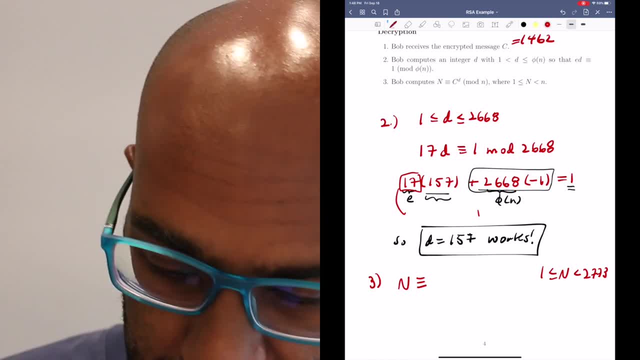 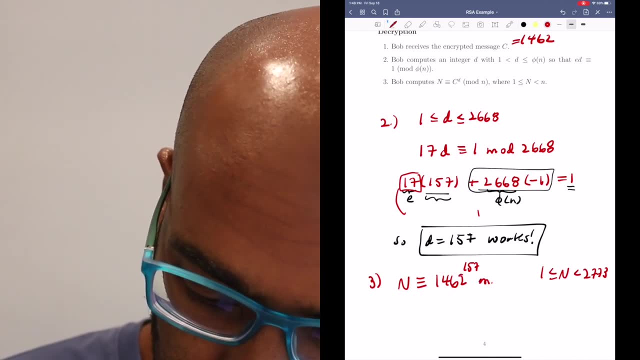 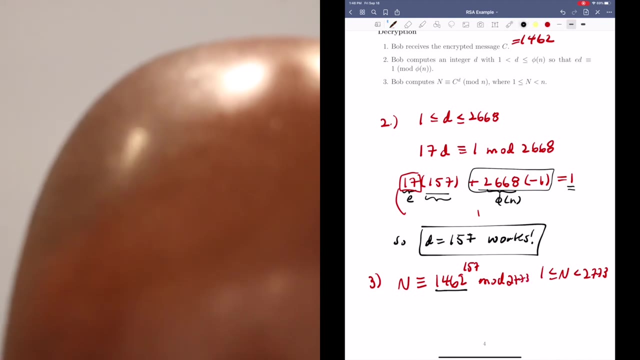 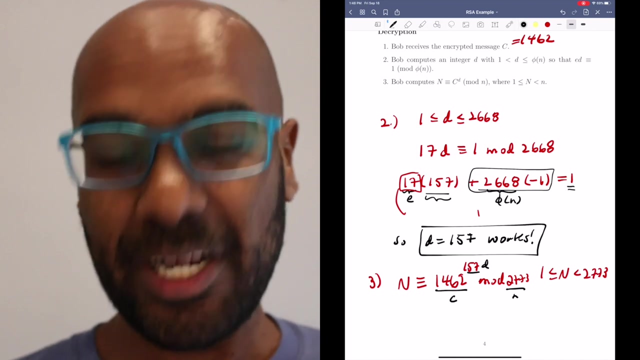 that n tries to take away the number of inches from these numbers. When you do that, you see how congruent to C, which is 1462, to the D157 modulo 2773. and again, this thing here is C, this is D and this was N. Now I'm going to leave it to you to actually try to do. 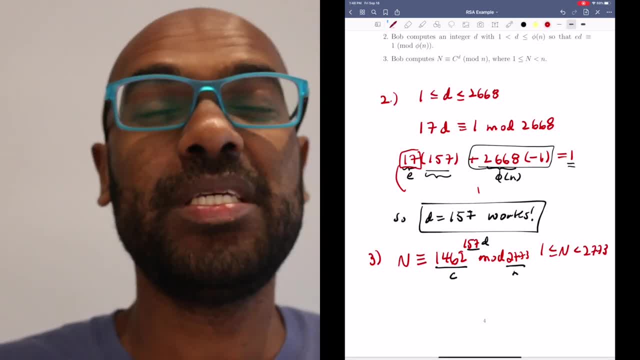 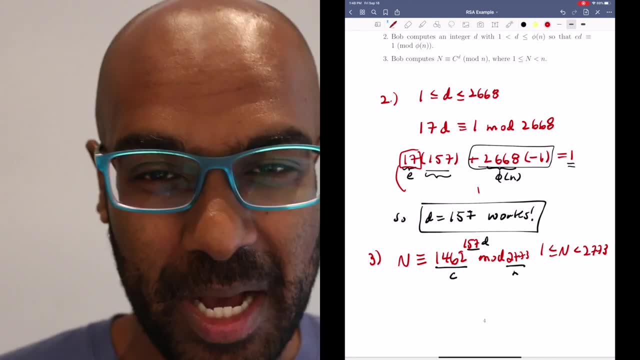 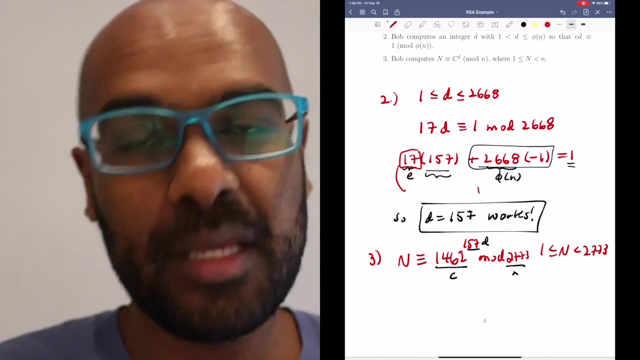 this computation. but if you do it- and I actually think you should actually do it- take 1462, raise it to the 157, compute mod 2773. you can take a step by step by taking 1462 and multiplying or squaring it, squaring that, squaring. 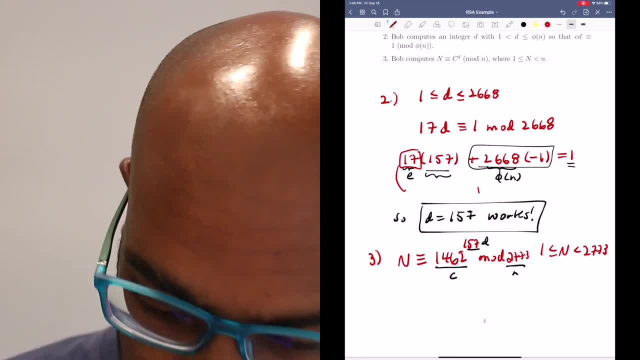 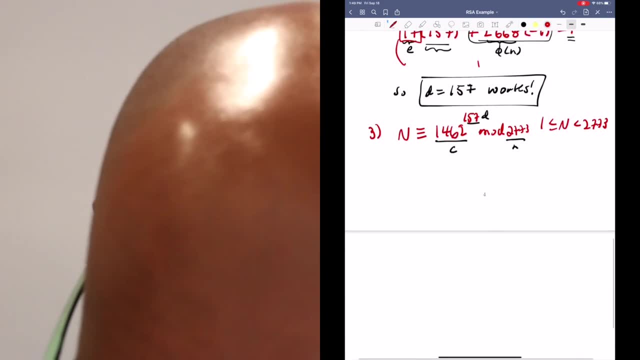 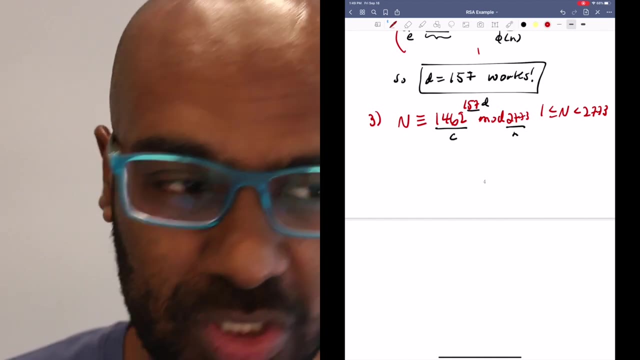 that, etc. multiplying by different things and seeing what you get. for example, you could write 14, so that's like one way of doing it. if you write 1462 with powers, there's also something that you can do to make things a little bit easier, which is actually really good in practice, Bob. 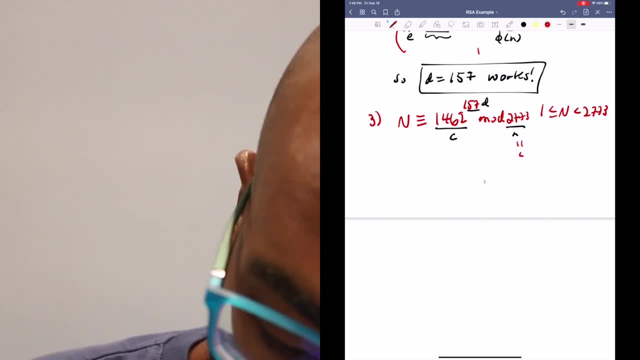 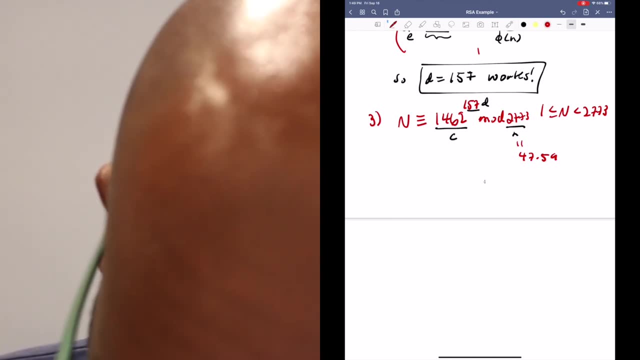 is the one who's doing this, and Bob knows that this number is 47 times 59, so what Bob can do instead is figure out what 1462 raised to the 157 is when reduced modulo 47, and also what it is when reduced modulo 59, and why that helps is this is a number.